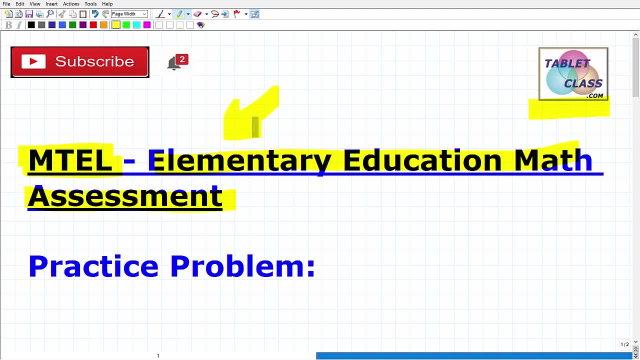 of this video and you can go ahead and check that out. But a little bit more on this particular exam. A lot of, oftentimes, not all the time, elementary educators, when they go to you know, start studying for their exams and they start thinking about the math sections on these particular assessments. they might, you know, it's logical to think that okay, I'm going to be an elementary teacher, So they're just. you know, the emphasis in terms of the math is going to be elementary math, right? 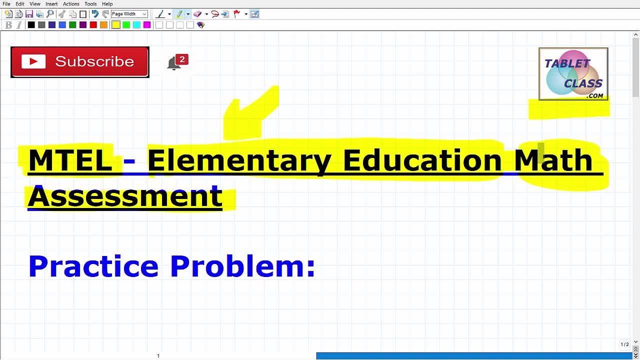 Right: Place value, decimal, basic fractions and stuff. So that's, it's logical to think in those terms. However, the reality is that the math that you need to know to do well in this assessment is far more than just elementary math. You need to know that those concepts as well- place value, et cetera- all the basics and foundational math that you're really going to be focusing on- But you're going to have to know a considerable amount of high school level math- okay, algebra, geometry, et cetera. So if math's not your thing, well, you need to warm up with it. 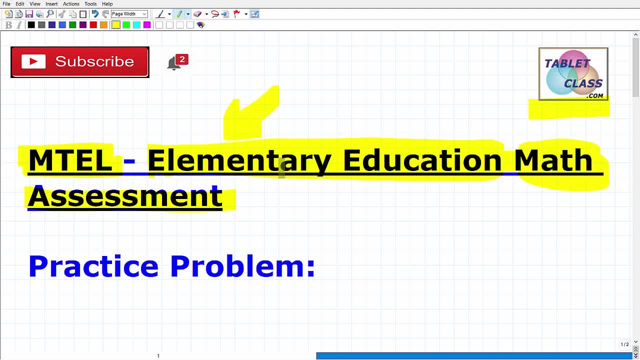 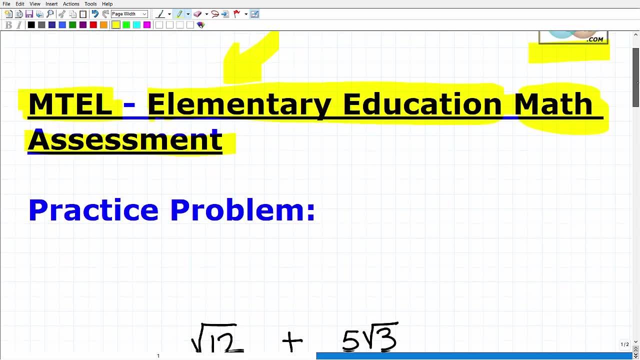 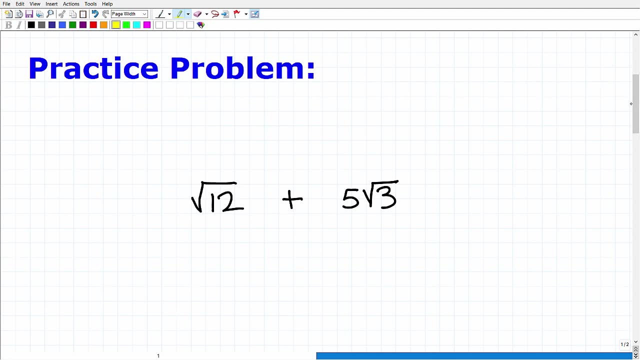 Do some studying and whatnot, So you're fully prepared for this assessment. So, with that being said, let me go ahead and show you the problem. Okay, And now? without the aid of a calculator, right? So definitely no calculators. That's what the whole idea here is. It's a problem that you should be able to handle pretty nicely. Again, if you're prepared, fully prepared, for this exam. All right, Now this is, I would classify This is a real basic level. 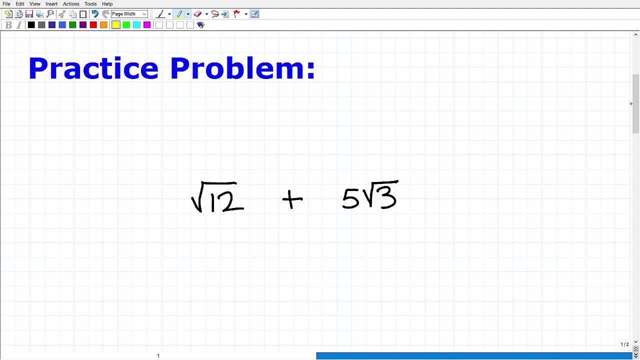 Algebra problem. Now, you've definitely learned how to do this And I'm sure a lot of you are like: oh yes, I remember these type of problems, but I can't remember exactly what to do. Well, that's, you know, a normal response, but that's not going to serve you well on the day you take this assessment. If you see a problem like this, you have to be absolutely certain what to do. Okay, Again, a basic, fundamental type problem. And here it is All right. So we have the square root of 12 plus five square root of three. I like you to simplify this. 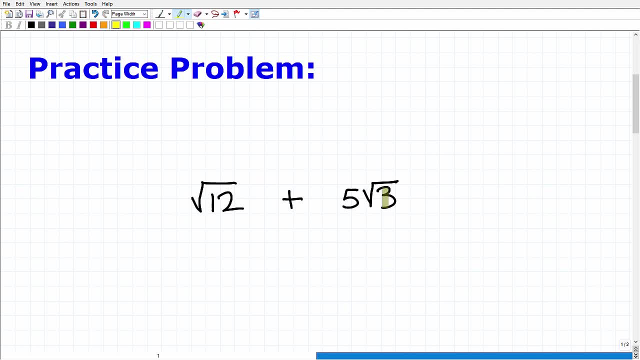 If possible, All right. It may not be able to be simplified, but if it is, if you're able to simplify it, simplify it, Okay, And write it using the square root, or we call radical notation, All right. So hopefully you understand what I'd like you to do in this problem. Definitely encourage you to pause the video. Don't go on, you know Google and search out how to do this problem. Just say you know, think about it for a second And obviously I'm going to solve it here, All right. So no calculators. The whole idea is not for you to. 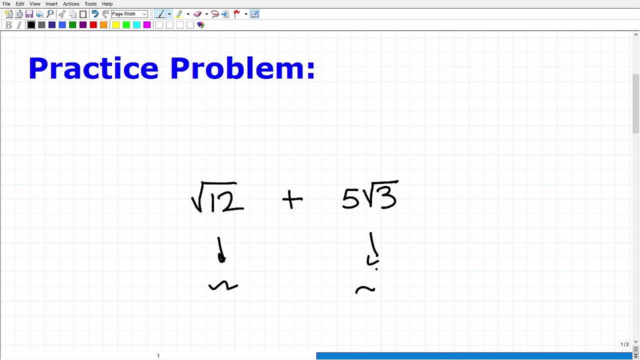 go in and get some sort of decimal value here. decimal value here, That's not what I'm looking for. Okay, I'm looking for your understanding of how to work with square roots or radicals, All right. So let's go into it now, And let's start with this: the square root of 12.. All right, So the thing here is this: Can I write the square root of 12 differently? Can I write it in a simpler form? And the answer is yes, you can. 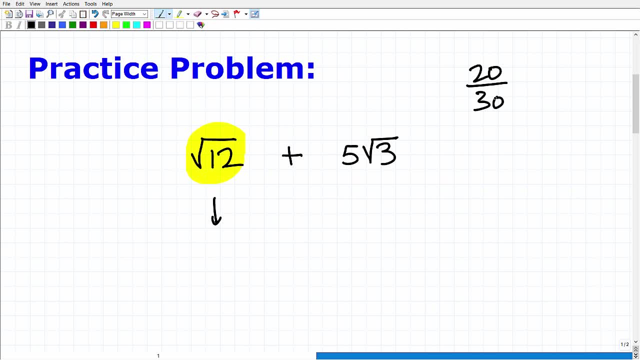 Just like we can write a fraction 20 over 30.. Okay, That is not in its simplest form, right? We can reduce that And its simplest form of that number is two thirds. Well, radicals, or square roots, have you know the same kind of concept associated with them. We can write these radicals in simpler forms, and we should- Okay, Shouldn't, leave a radical like non-simplified if it can be simplified. It's like writing a fraction 20 over 30, where you want to write it as simple as possible. 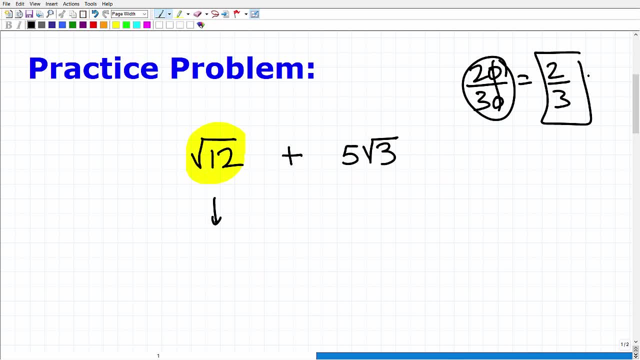 It has two thirds in its fully simplified manner. So, when you're studying square roots, this is kind of the beginning points in terms of working with square roots. So let's go ahead and talk about how we simplify a radical like this Square root of 12.. Okay, So the square root of 12, I can think of, and I want to think of, as the square root of its factors, Right, So there's a bunch of factors, Not a bunch, but there's, you know, one times 12,, six times two And oh, we have four times three. 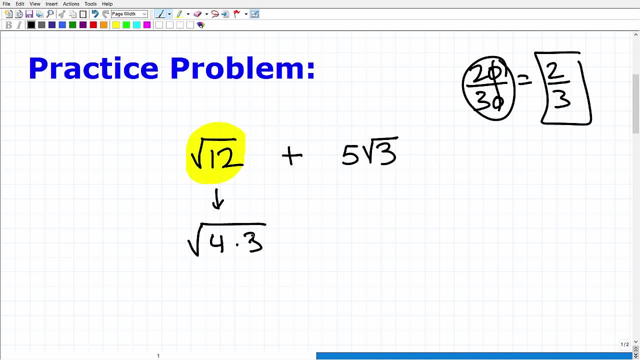 So four times three is a nice way to nice pair of factors of 12.. Okay, So the square root of 12 is equivalent to the problem, the square root of four times three. Right, Just intuitively you can see why that's the case. But now you might be interested in this little four Right So numbers that we call these perfect squares: four, nine, 16,, 16,, 25,, et cetera. 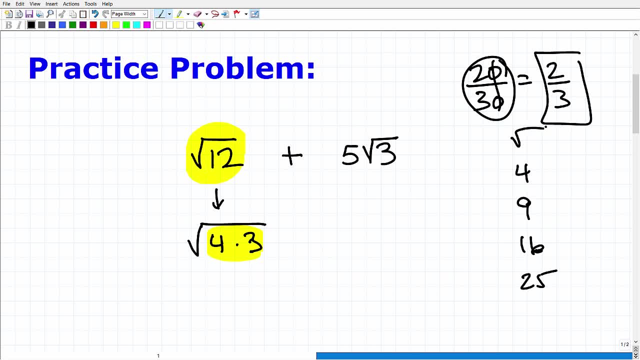 So these are nice numbers when we're talking about square roots, Right? So why is that the case? Because if I said, hey, what's the square root of these numbers? You would immediately, without your calculator, be like: oh, that's easy, That's two. This, by the way, these are all positive, negative, But that's another discussion. But this is two, This is three, Oh, this is four, This is five. So when we square these nice little numbers, we get these numbers and we can find the square root. So these are called perfect squares And we're dealing with square roots. 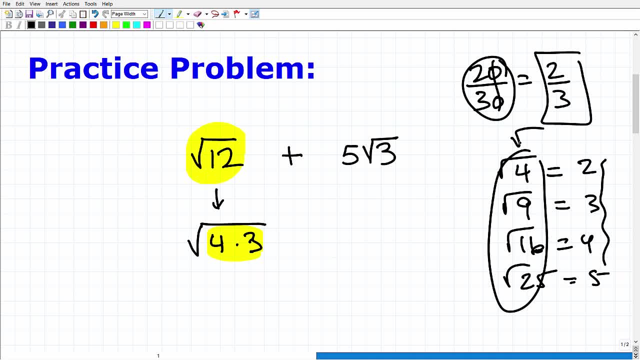 And problems like this. you're always on the hunt for these kind of numbers because they come in very handy. So the square root of 12 is the same thing. It's a square root of four times three. Now I'm like, well, this is a perfect square. It's inside, It's part of, it's a factor of this number. I'd like to maybe get it out of here or do something with it, And the good news is you can. Okay, So the square root of four times three. I have this one big radical here. I can write this this way: Square root of four times three. 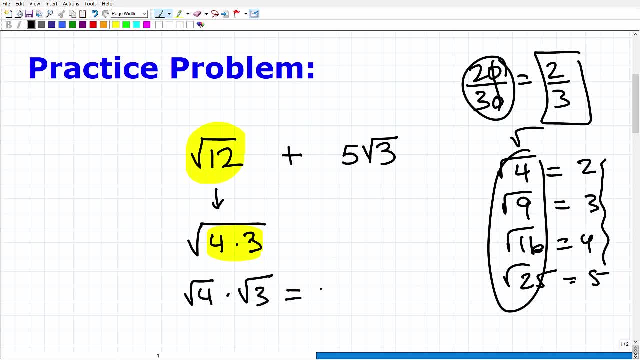 Square root of four times the square root of three. That's the same thing. Or this is another way of writing: a square root of four times three. Okay, This is what I was kind of getting out of here, Right? So you need to know this, These properties, these laws of how to work with square roots- And this is a major one. Okay, So we can rip factors apart into their own separate little square roots, like this. Now, what's the advantage of doing that? Right, Go ahead. 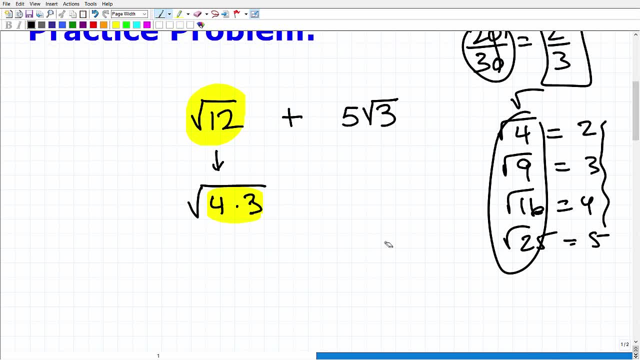 Give us some room here. Well, knowing that, I could say: okay, this is a square root of four times the square root of three. How does this come in handy? Well, at this point here I can now go ahead and find the square root of four. That's going to be two, Right? So we'll write this as two square root of three. Now, technically it's positive, negative. We're just going to just leave it as two square root of three. So the square root of 12 is now. we kind of wrote it in a simpler manner. 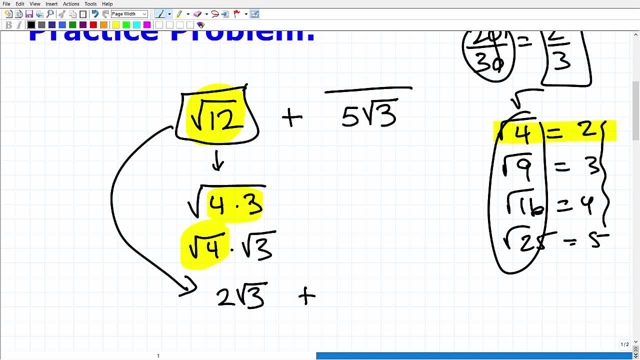 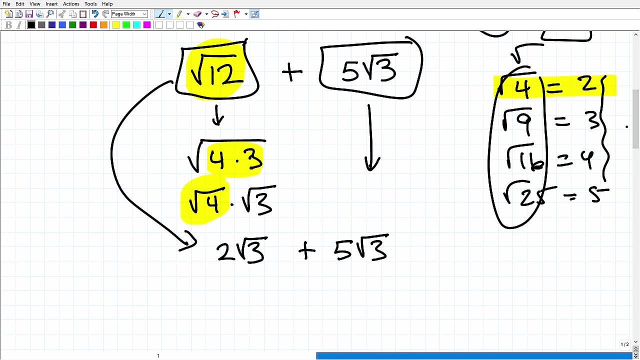 Two square root of three. Now let's bring in the rest of the problem. Okay, That five square root of three. Write that a little bit better. Okay, So now at this point- and by the way you know, hopefully you know anytime you think you can answer the question, then you know you should just pause the video and answer it Like: okay, now I know what to do, Then go ahead and solve it, All right. 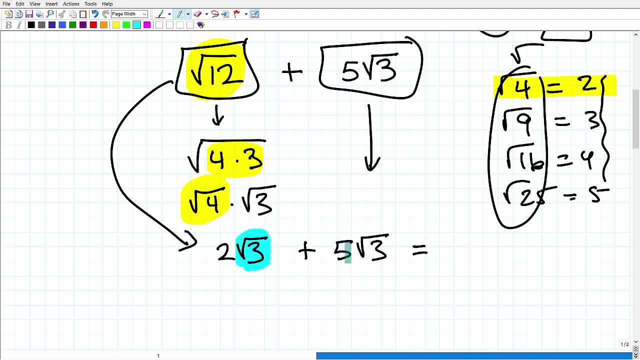 So here we look, that we have two square roots of threes here and we have five square roots of three right here. This is very much like basic algebra, like two X plus five X. Okay. So what's the answer here? This is seven X. We have seven X's all together. So when you have the exact same radical here, square root of three, square root of three, it could be whatever, And we're adding or subtracting. Okay, Adding or subtracting, You're going to treat it. 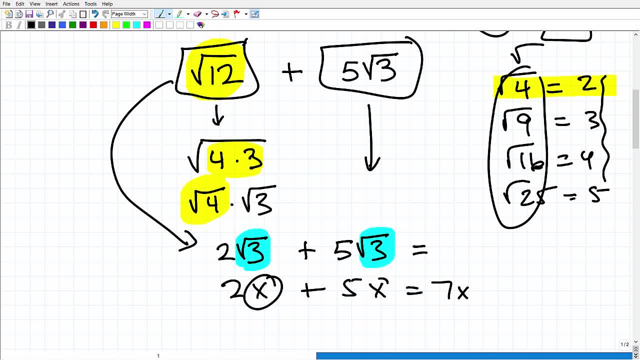 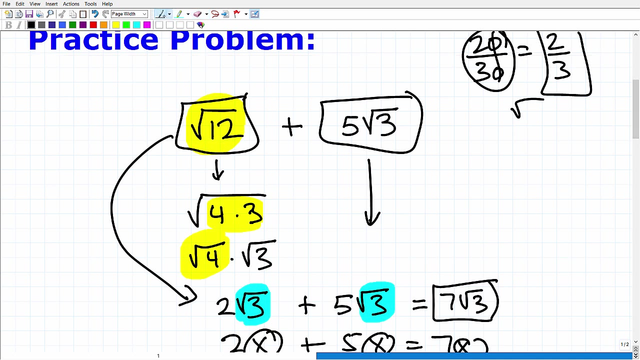 Exactly like like terms in algebra. Okay, How we identify like terms. So here the answer is going to be seven square root of three. All right, That is our final answer. Okay, So if you understood that, got that right And you're like no problem, That was easy, You know, you know kind of boring, I wanted a more challenging problem. Hey, then, you know you want to. you know, get into my math course or go, you know, look for other problems. 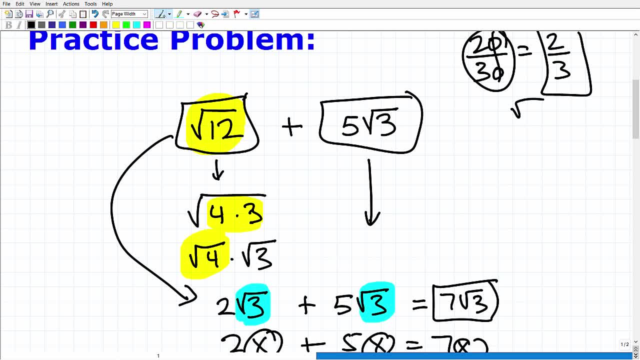 They're more challenging, But this is really, you know, fundamental stuff. Of course, if you were struggling and you didn't really remember any of this, don't panic, Just use it as feedback. But when we're talking about square roots, you need to know how to simplify them, Okay, That's what we just kind of did right there. And then you need to know how to add and subtract them. We talked about a little bit about that. Then you need to know also how to multiply and or divide, Okay, And then there's some things called rationalizing as well. 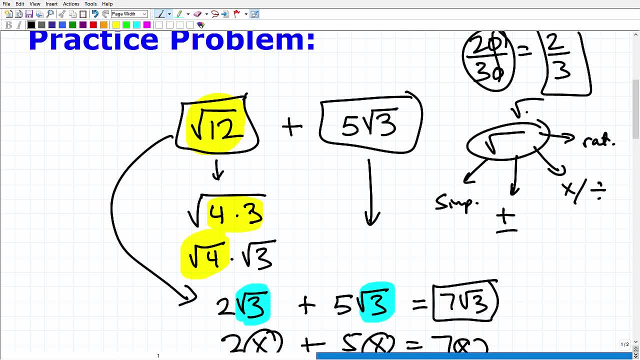 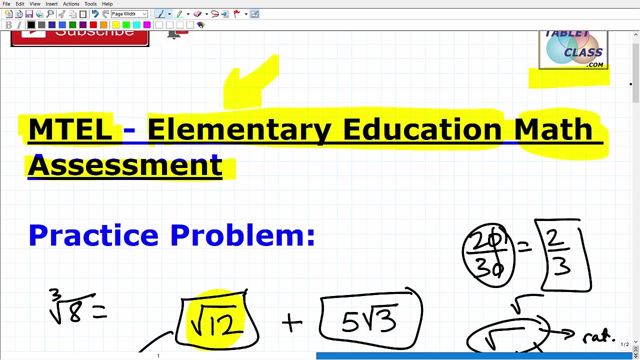 And so we can kind of go down a whole path of different things we need to know about square roots, radicals, And then you can kind of get into other things that you know: cubics, you know like not square root, but you can have the cube root of eight, etc. etc. So again you can go down many tangents. But all these things you should have a good grounding in, you know if you're going to be fully prepared for the MTEL, elementary education math assessment. Okay, These are professional assessments, All right. 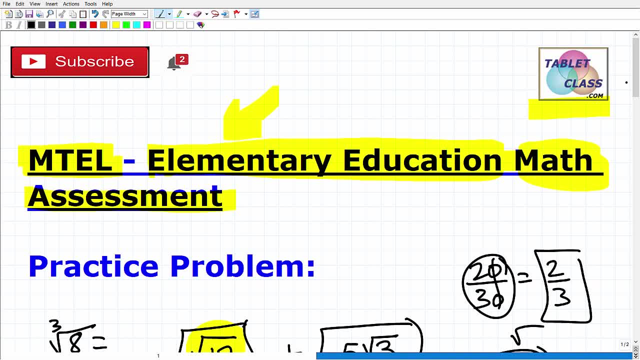 And again, the main point that I was trying to make here is that you're going to be seeing math. That's just not all elementary level stuff. Okay, You got to know your place value. You got to know basic number concepts and all that kind of stuff. You know. you know at the elementary level. you know all the way up to the fifth grade. you know that's a lot of mathematics. You know you go into the sixth grade you're handing those students off and from middle school math and then they're going to get ready. 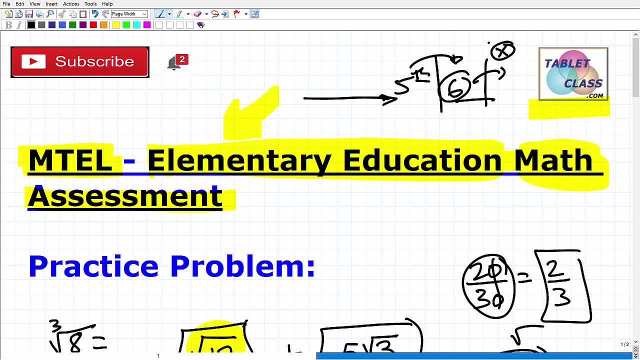 For high school. I taught middle school and high school And I was when I used to get you know great students. you know, in ninth grade I was like man, you know all these teachers did a great job. all back here you're really, you know, setting these students up for success for middle school. So it's like a baton right And you got to. you know, get these students ready for you know things that they're going to be facing in middle school. And you know middle school. you know you're doing basic algebra and geometry. you know you can have accelerated students taking full on algebra one or 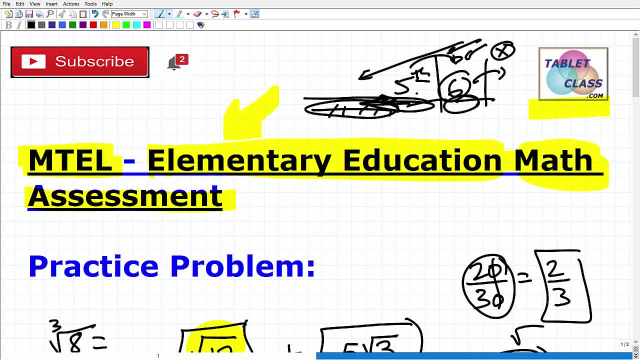 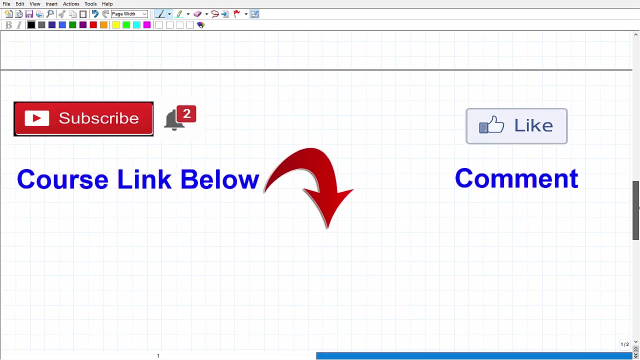 even geometry courses. So that means you're going to have to be doing a lot of that. those you know, prepping those concepts you know at the elementary level, All right, so I think I- hopefully you know- made my point that you're going to need to know more than elementary level math. Again, a lot of different ways you can prepare for it, But the main idea is to have a plan, Okay. So, again, it's going to wrap up this video. I'm going to leave a link to my test prep course on this assessment in the description. check that out. 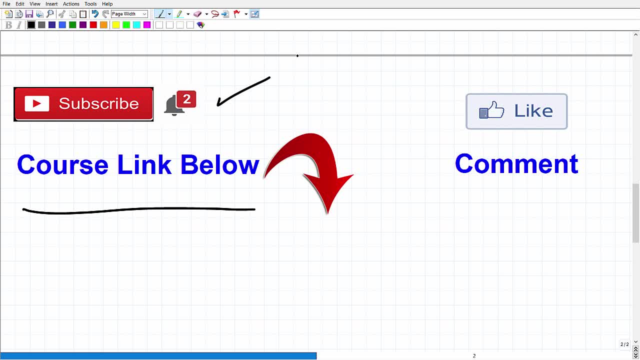 Also, I'm posting content all the time, almost. you know, just many videos per week. I love teaching math And so I already have hundreds and hundreds of videos on my YouTube channel. So if you like my teaching style and you know you're, you can learn from me. please check out. you know all the videos are on my channel. I kind of organize them in various playlists, So hopefully that helps you out. And you know, becoming a subscriber is even better because I'm posting new and fresh content all the time And if you enjoy the video, definitely appreciate it. 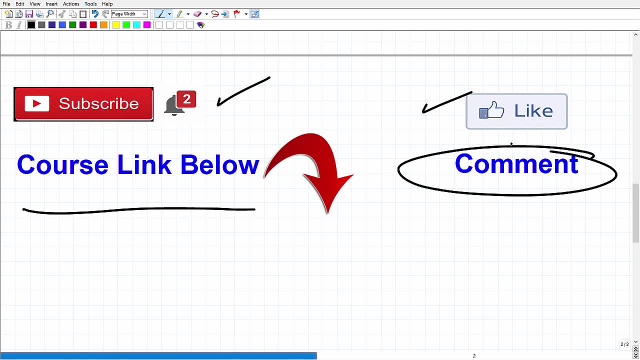 Thumbs up and leave me some feedback. What's your kind of career path? you're going from high school to college, to teaching, which is a classical approach, And that's great because that means that, hey, you know, you knew, you know early on that you wanted to be a teacher. But maybe you're one of these folks that you know, or you know 20 years and you know as a real estate agent or business or some other career, and now you're becoming a teacher. There's a lot of teachers that are 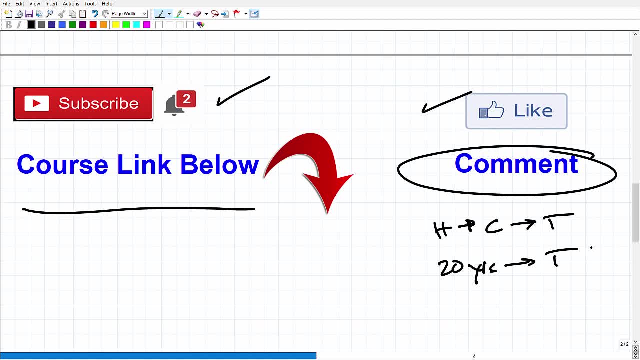 that you know come into education from other careers, And I think both are great paths. especially nowadays, there's so many different ways you can become a teacher, And I think that is super smart, for the system to be set up that way, because we just need teachers, we need a lot of teachers, we need great teachers, And so, whatever you know path that you've taken, it's never too late to, you know, make an impact. Okay, so, whether you've you know, you don't have to be. 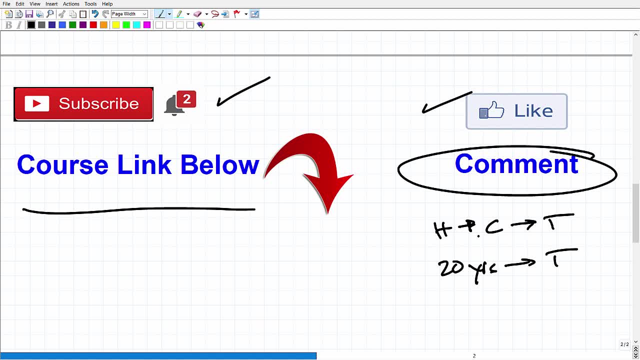 young, young, young to start teaching and whatnot. but the one thing i will say is this: even if you're you're you're starting teaching at 40 or 50 years old doesn't make a difference. the one thing is just remember when it comes to teaching, all right, irrespective of where you're starting.